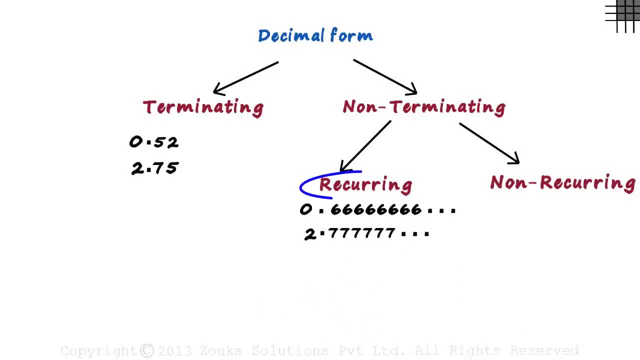 seven, seven, seven, seven and so on is a recurring, non-terminating decimal, since it does not end and the number seven is repeated indefinitely. But does it mean only one digit can repeat indefinitely? No, Look at eighteen point five, two, five, two, five, two and so on. Here, five. 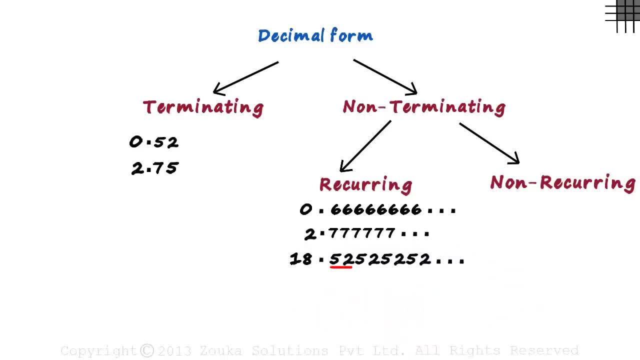 two is repeated indefinitely after the decimal point. Since five, two is repeated indefinitely and it does not end, it's called non-terminating recurring decimal. Also, does it mean that the repeating part starts immediately after the decimal point? No, Let's look at seven, point six: five, two, three, two, three, two, three and so on Here. 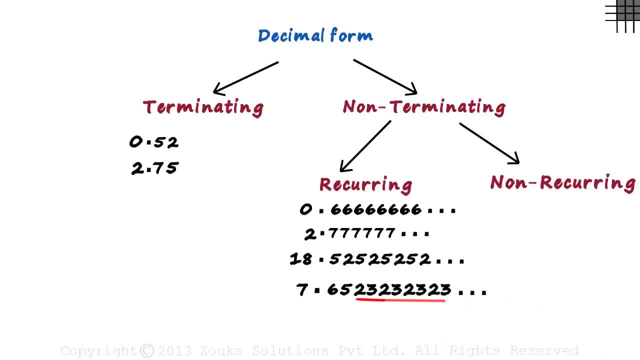 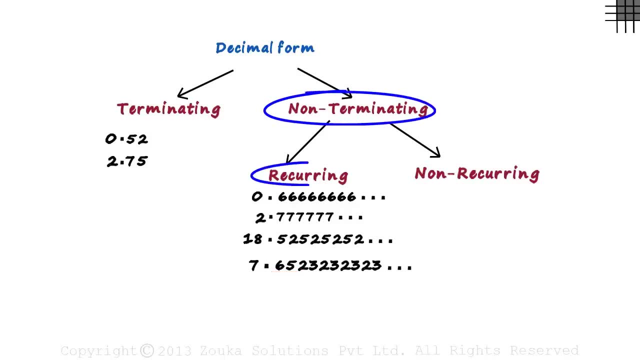 the number two, three is repeated and goes on forever. But the decimal part starts with six, five. Even such numbers are classified as non-terminating, non-terminating recurring decimals. The non-terminating recurring category forms a very important category in decimal representation. 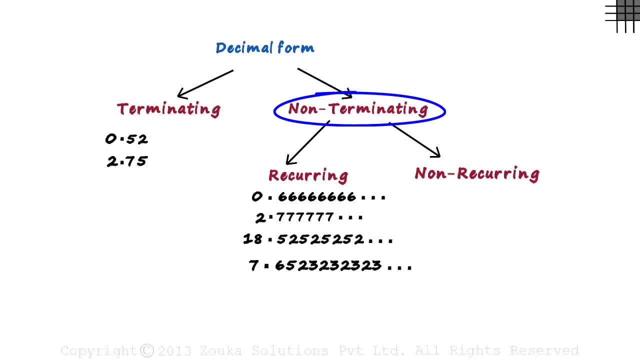 We will look at just this category in one of our videos. Non-terminating- non-recurring simply means that the number does not end and the digits after the decimal point do not have a specific pattern. The best example would be Pi, 3.14159 and so on. 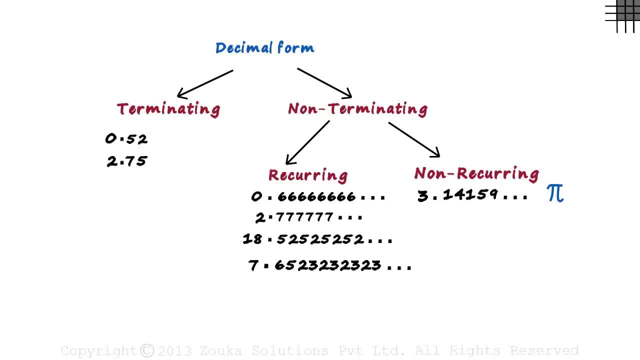 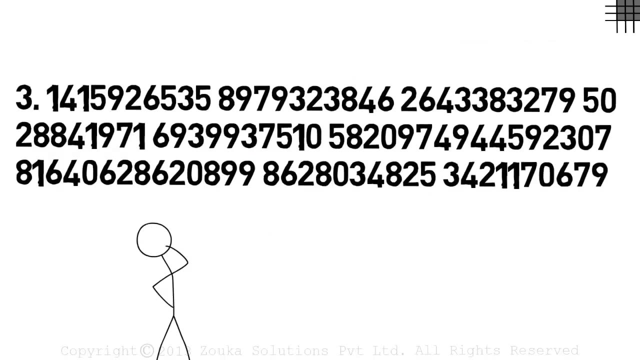 The number does not end, and even if you have 100 digits after the decimal point, you will not find any pattern or any indefinite repetition of digits. Here's the value of Pi up to 100 digits. Look at the digits carefully. You will see no pattern whatsoever in here. 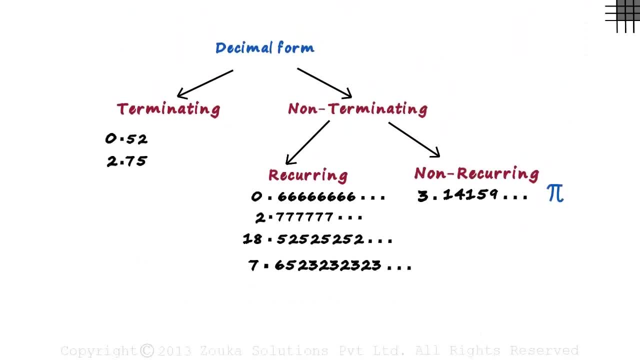 That is the reason it's called non-recurring. You can even form non-recurring decimals on your own, Something like 6.20300300.. 3000 and so on. There you go. You will not find any pattern here. 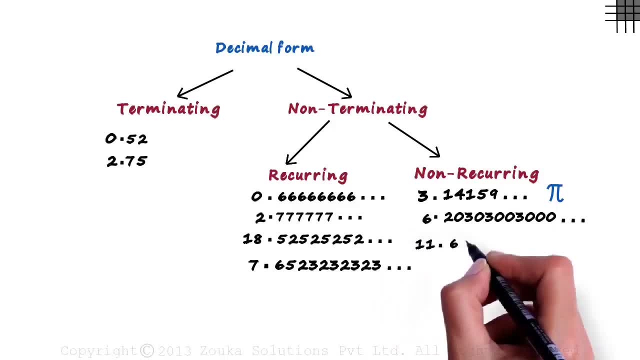 Or maybe something like 11.671711711171111 and so on. You take any two digit number, like 30, and write it by repeating the units digit. again, The units digit is zero. So we write a 300 and then we add the units digit.